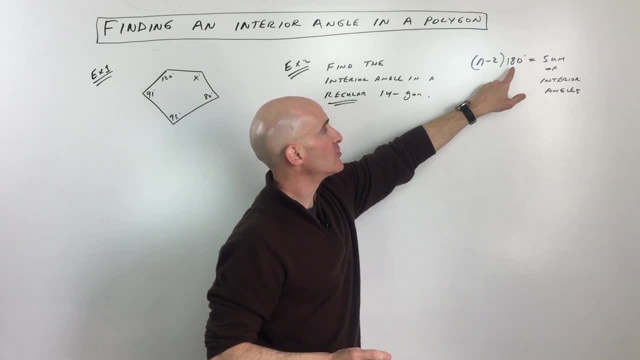 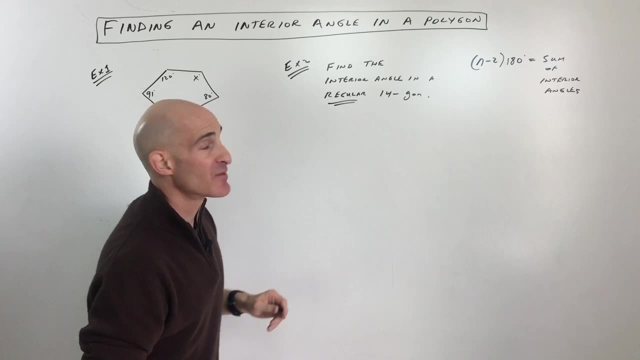 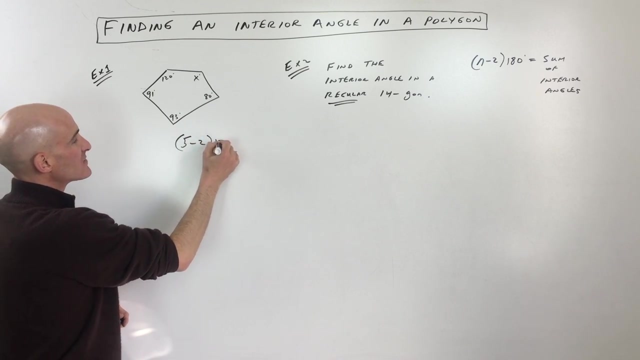 And the formula that we want to use is this one right over here: It's: n minus 2 times 180 equals the sum of the interior angle. So all the inner angles added up, Okay, that's going to be that total there. So here you can see, we've got five angles or five sides, either one. Five minus two times 180 equals what? Well, that's three times 180, which equals 540.. All these angles have to add up to 540.. So let's make an equation: 91 plus 120 plus x. 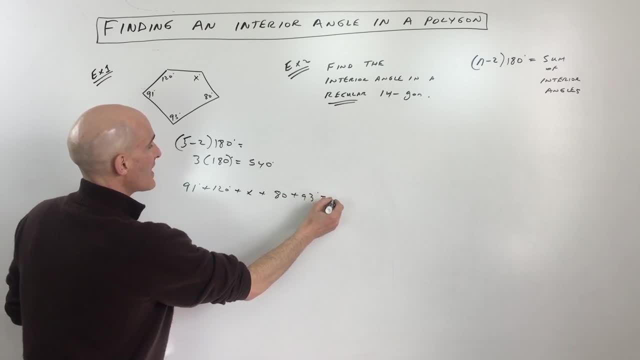 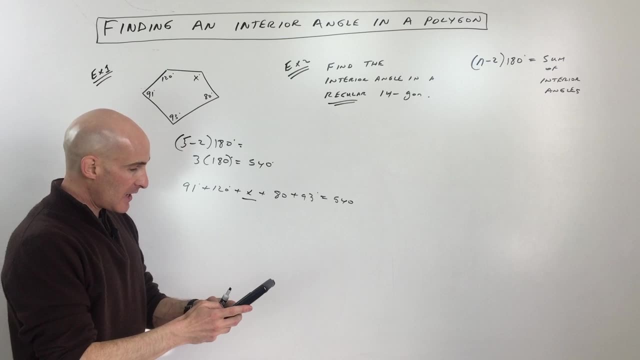 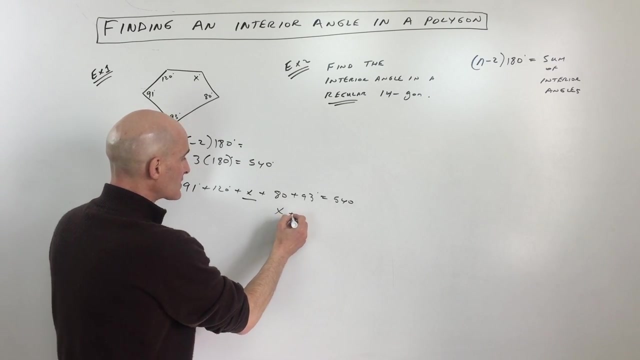 Plus 80 plus 93 has to add up to that 540.. So all we need to do now is solve for x, and we've got it. So let's go to the calculator: 91 plus 120 plus 80 plus 93. That comes out to 384.. So we have: x plus 384 equals 540.. Just subtract the 384 from both sides, Right, And we've got it. So 540 minus looks like 156 degrees. So 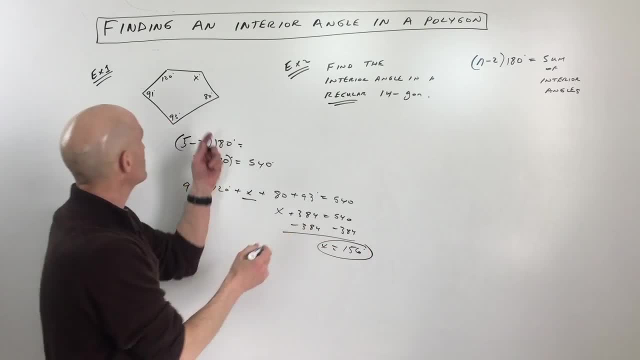 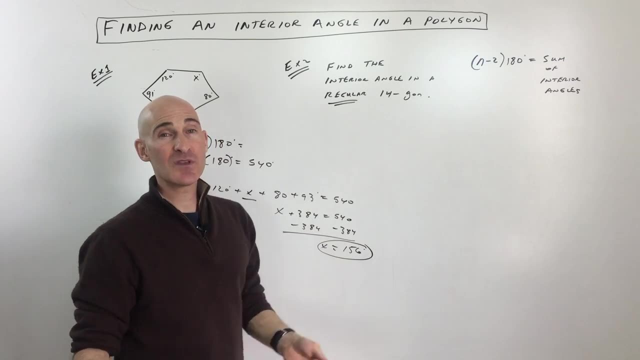 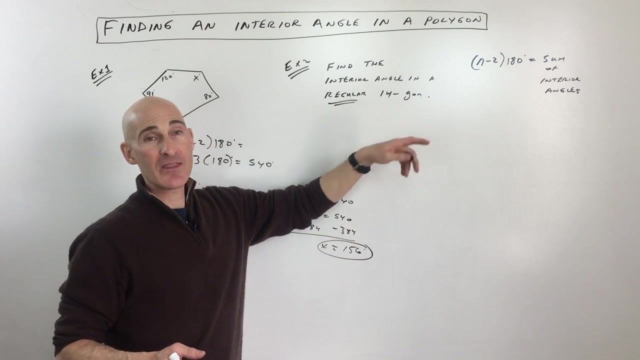 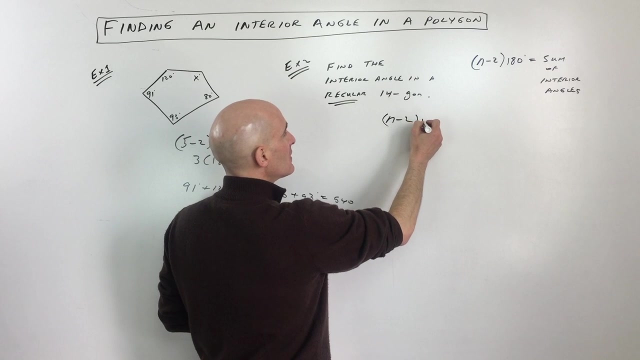 that's the measure of that missing interior angle, this one right here, Okay. so the example number two says: find the interior angle in a regular 14-gon. So what does it mean when they say regular? It means all the angles are the same, Okay, and all the sides are the same length as well. But if it's a 14-gon, that means it has 14 sides or 14 angles. So what we're going to do is we're going to do this a couple different ways. We're going to do n minus 2 times 180.. Okay, in this case it's 14.. So I'm going to put 14. 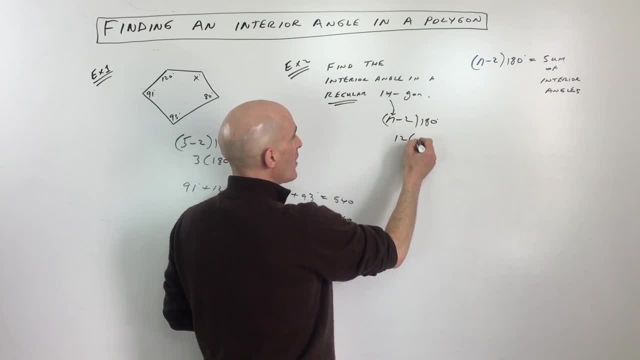 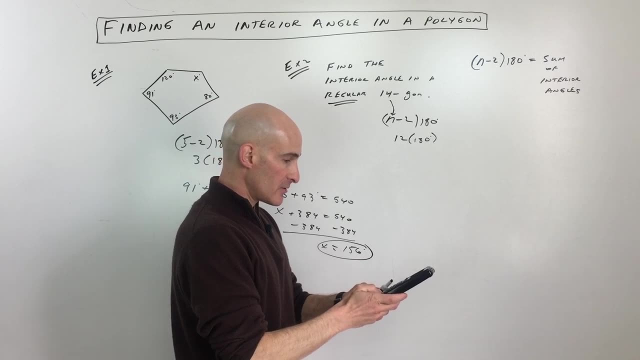 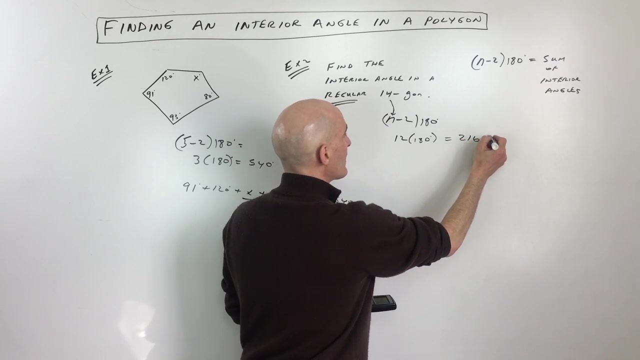 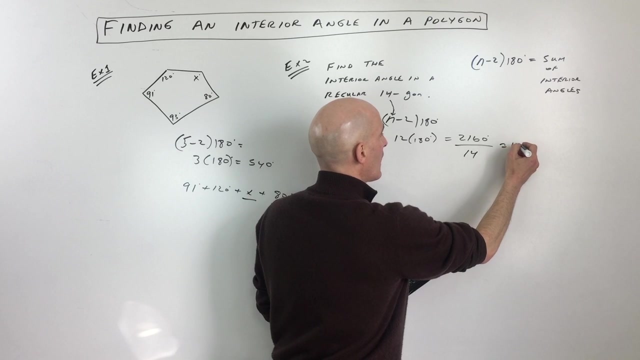 right there. So we've got 12.. 14 minus 2 is 12 times 180. That's going to give us the sum of all the interior angles. So if we do that, we'll go to the calculator here: 12 times 180. That gives us 2160.. But we just want to find the measure of one angle, So we're going to divide by 14, since there's 14 of them. Right, Okay, so that was pretty easy. It's about 154.3 degrees. The other way to do this problem is you can use 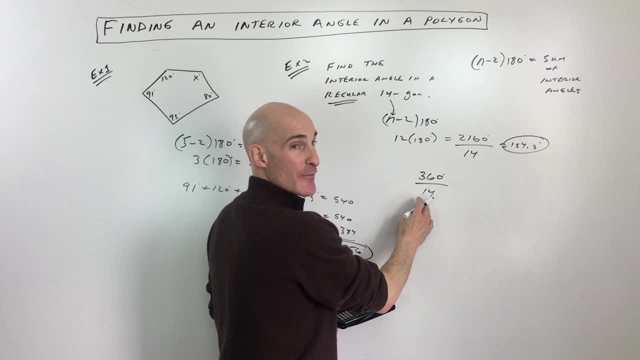 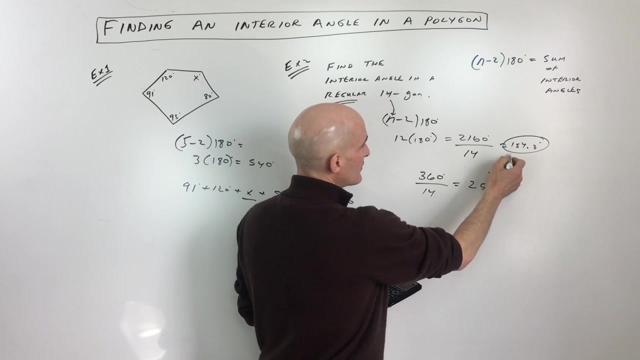 the formula 360 divided by n or divided by 14.. This will give you the measure of the exterior angle. Okay, because all the exterior angles always add up to 360 in a polygon like this. So basically, the exterior angle is coming out to 25.7.. And one thing you'll notice about these two: